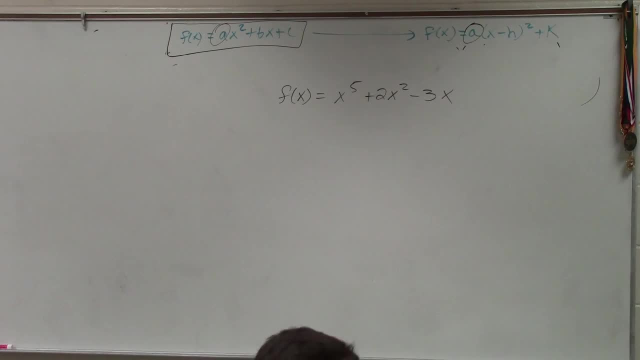 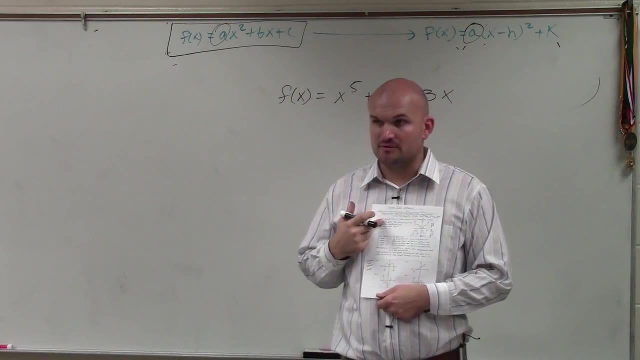 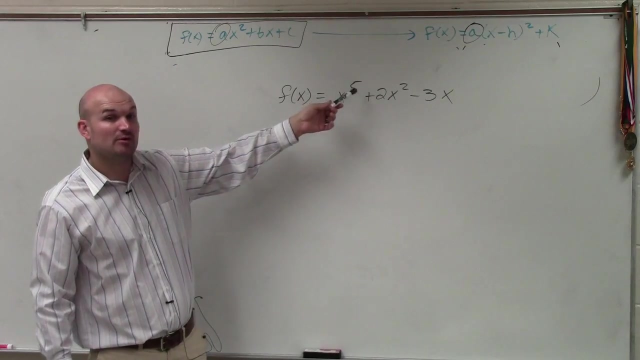 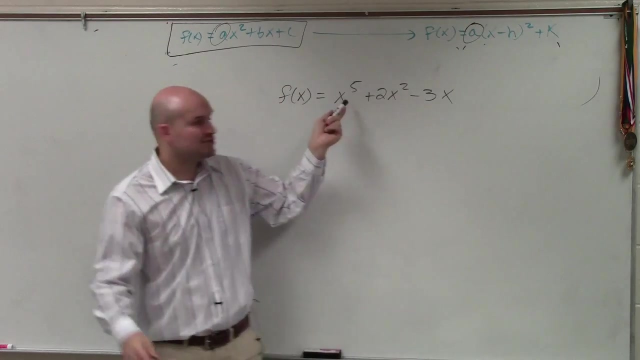 So to determine the n behavior, basically on your guys' notes, on your n behavior on the front, I again went back over the definitions of degree and leading coefficient. The main important thing to do that is you've got to have your polynomial in descending power, meaning you have to have the highest power first and then keep on going down and down and down. right, So if these were like reordered, you'd make sure- always make sure- that this is in the front, okay Then of that term that has the highest power. you've got to have the highest power in descending power. 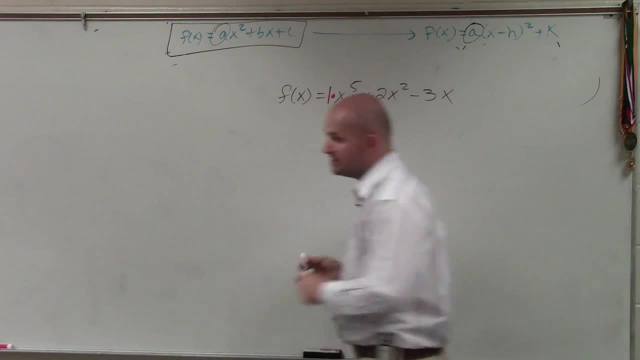 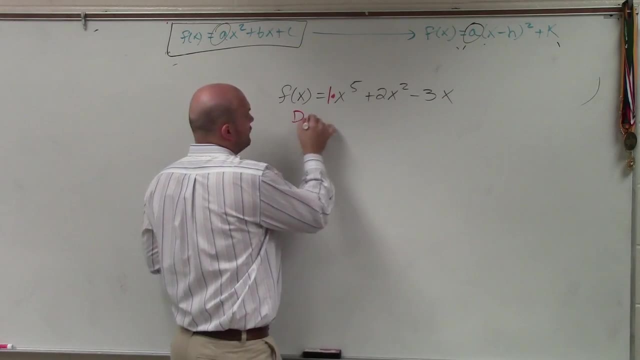 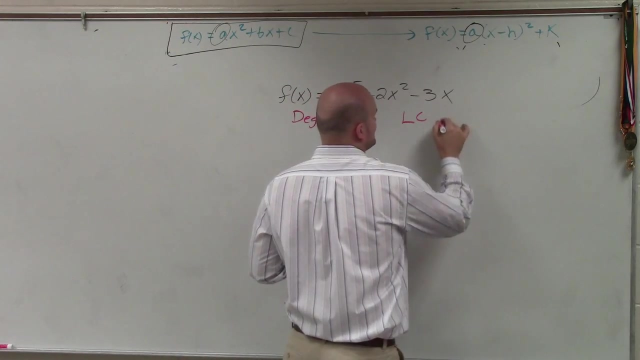 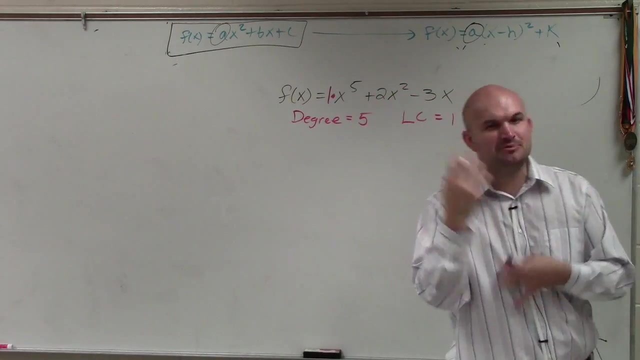 There is a coefficient, which we call the leading coefficient, which in this case is one. So a lot of times, when determining n behavior from a polynomial, I like to just to remind myself what is the degree and what is the leading coefficient. The degree in this case is five and the leading coefficient is one. okay, So there's no harm in doing anything like this. Just write them down. That helps you remember. Now the next thing is we need to understand: is my degree? 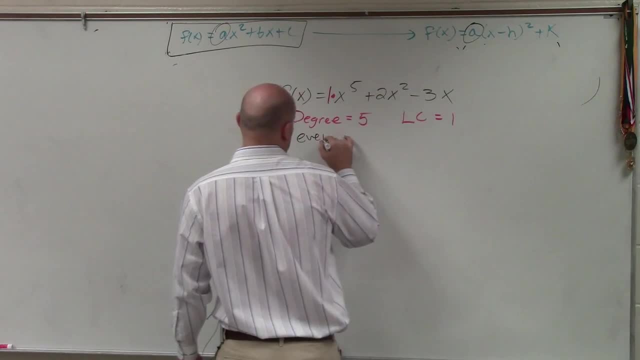 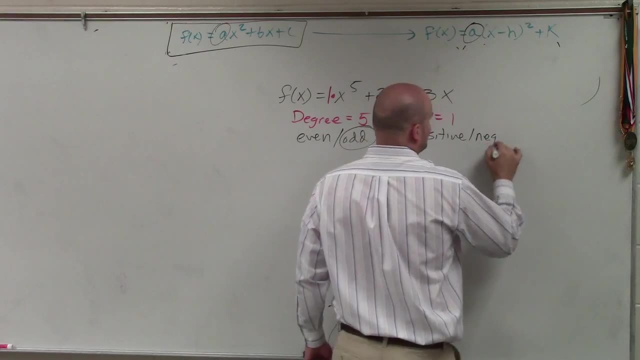 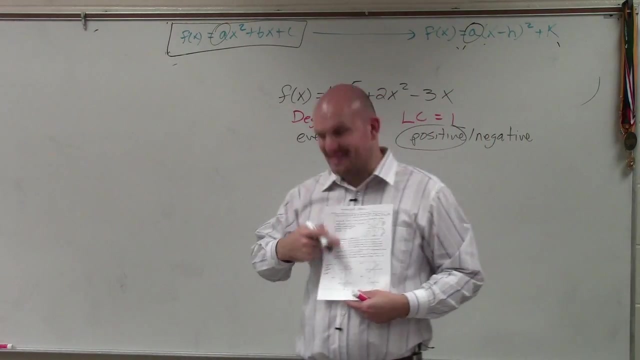 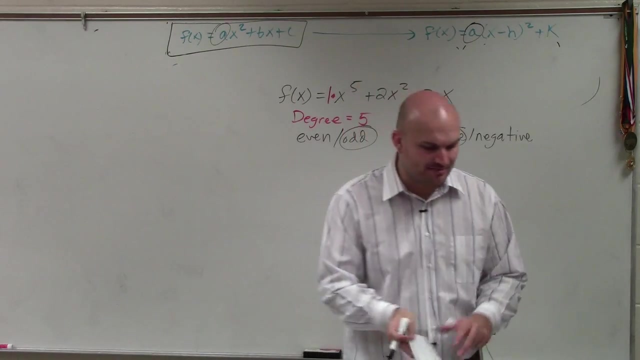 even or odd. It's odd. Is my leading coefficient positive or negative? So since I know it has a positive or negative, you guys could use this, which I think is kind of confusing. I just like to kind of think about this and know what it looks like. What is the general n behavior of a graph that has an odd? 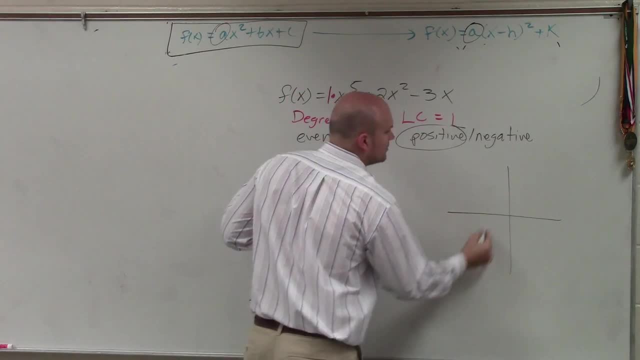 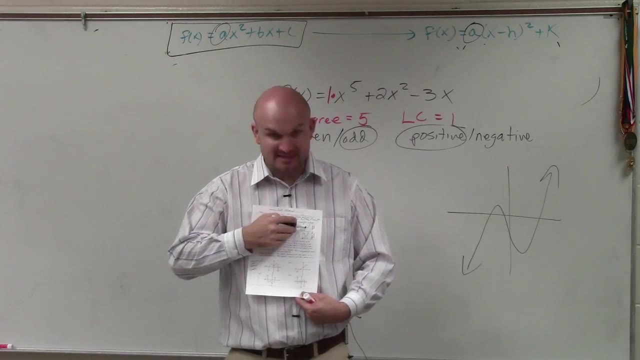 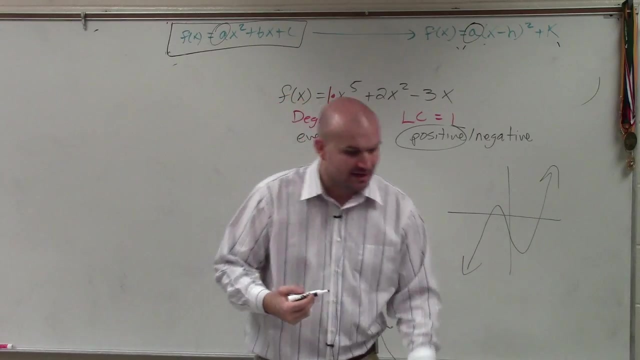 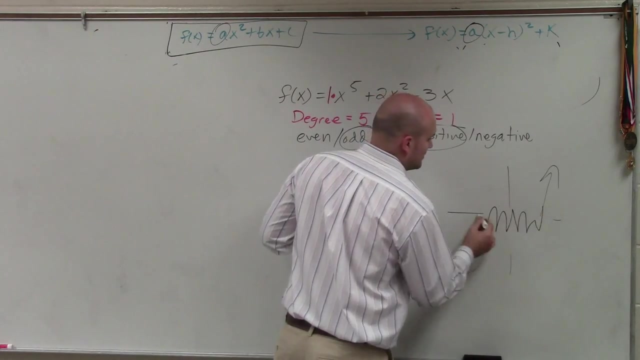 degree and a positive. Well, it's going to look something like that. As you guys can see, I did a representation of that up here. The degree is odd and the leading coefficient is positive. So you can see, the graph looks something like that In reality, though, we don't really know what the graph looks like. The graph could look like that, The graph could look like this. It doesn't really matter what the graph looks like. The main important thing in n behavior is it tells you what the graph looks like. 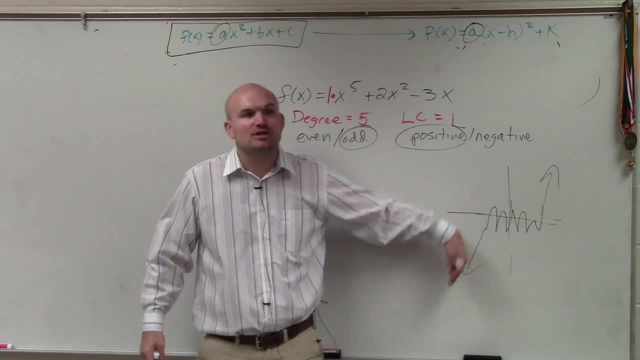 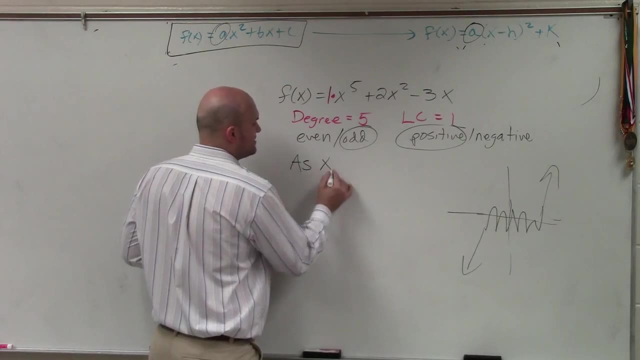 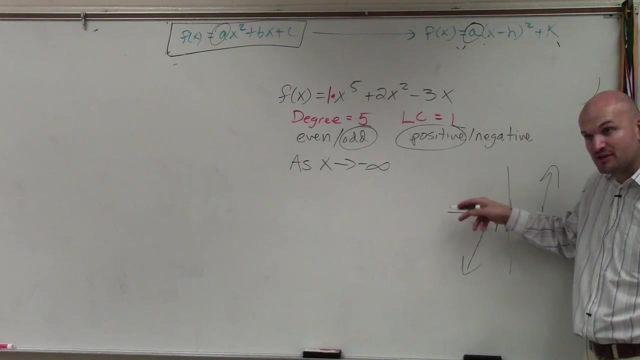 What the n behavior graph does. What is going to continue As you keep on going to left? where is the graph going to go? All right? So then, as I mentioned, you always write the same as forward, As x goes to negative infinity. where is this graph going, Up or down?